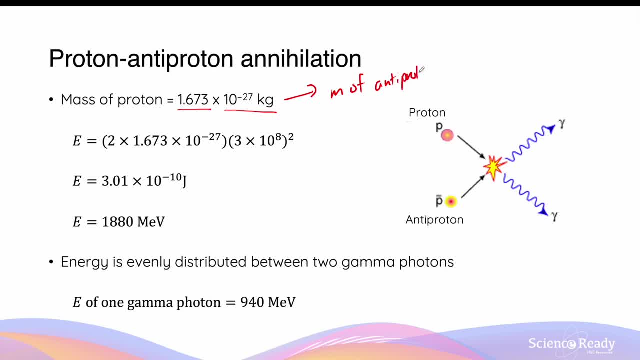 of the antiproton. Remember that the antiparticle has the same mass but the opposite charge as its particle. When the mass of the proton and antiproton are transformed into energy, we need to include the mass of both particle and the antiparticle, which is why we multiply the 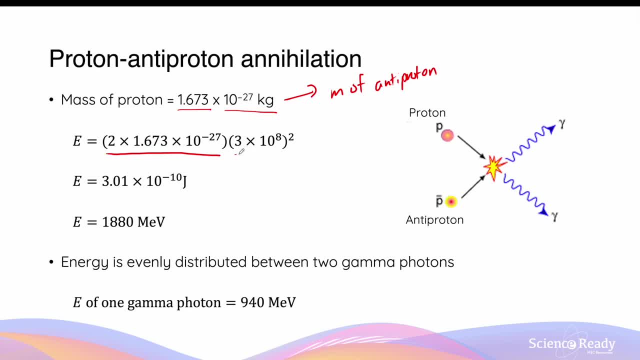 by 2.. Since the mass is in kilograms, we can multiply this by c squared in minutes per second, and this gives us 3.01 times 10 to minus 10 joules of energy altogether. We can convert this into mega electron volts by dividing by 1.602 times 10 to minus 19, and then further dividing it by a. 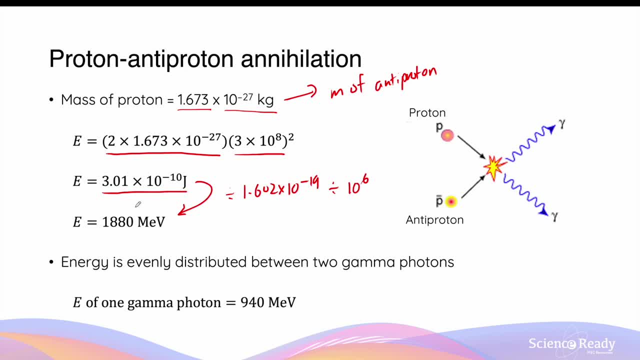 million, to commit to mega. This amount of energy, whether it's in joules or mega electron volts, are shared evenly between two photons that are produced from this annihilation process. So the energy of a single gamma photon can be calculated by simply dividing the total energy, which is 1880, by 2, and that is 940 mega electron volts. The annihilation 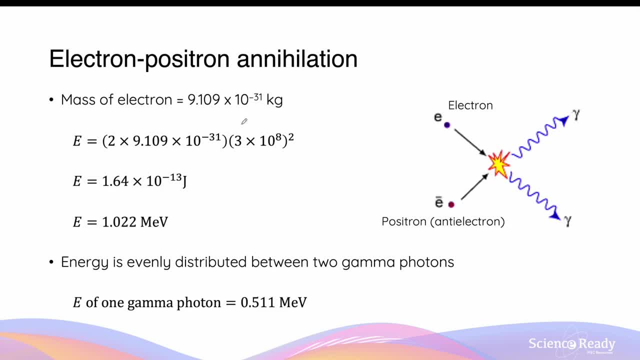 between low energy electron and positron behaves in a very similar manner. The energy of the photons that are produced can be calculated by considering the combined mass of the electron and the positron, which is a common name given to the anti-electron, The antiparticle of an electron. When we multiply the mass of the electron by 2 and times by the 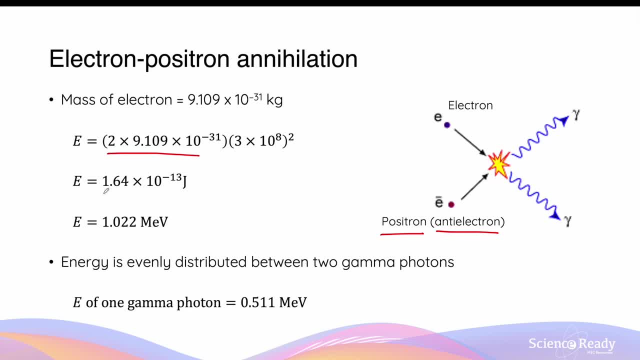 speed of light squared, we'll get the energy that's produced, which is 1.64 times 10 to power, minus 13 joules. Again, we can convert this into mega electron volts. Whether it's in joules or mega electron volts, this energy is again shared between the two identical photons, So the 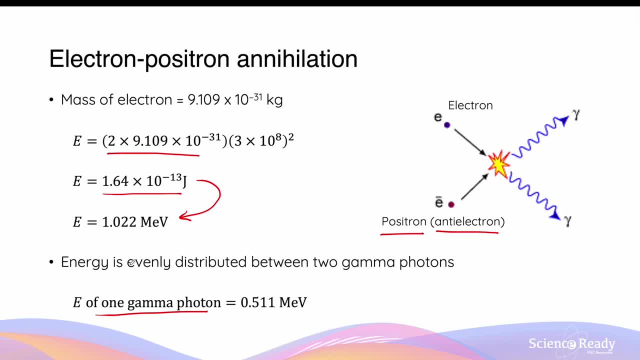 energy of one single gamma photon can be calculated by dividing the total energy by 2, which yields a value of 0.511 mega electron volts. In both examples of low energy annihilation, the particle and its antiparticle are completely transformed into energy in the form of two photons. The 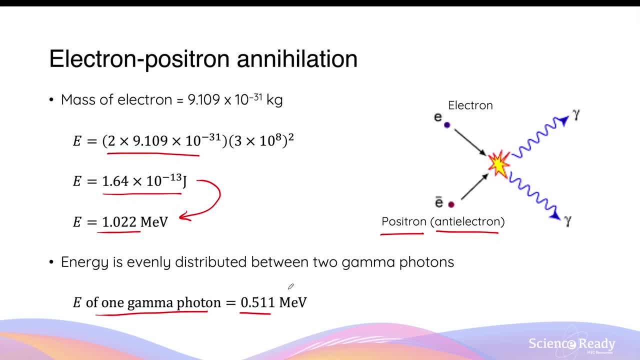 kinetic energy of these particle and antiparticles prior to the collision are not included in the calculation, as they are relatively negligible compared to the energy derived from the mass. It is also important to note that the starting mass of the particle and antiparticle will